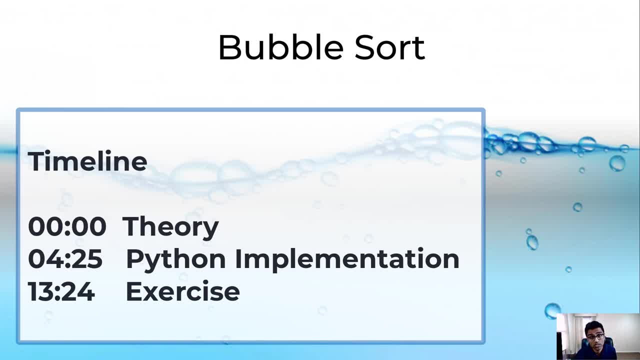 We will be discussing bubble sort in this video. As usual, we'll have some theory, then we will implement bubble sort in Python and at the end I have an interesting exercise for you to work on, so make sure you watch till the end. Why sorting is needed in first place When you're developing big projects such as. 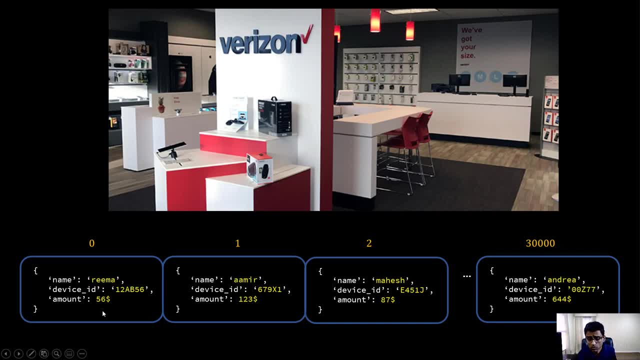 let's say you are building a system for wireless store where in your computer you might have so many transactions. let's say you have 30,000 transactions and I want to sort this transaction by the amount. I want to know who bought the maximum amount of inventory from my store. Sometimes I might want to sort 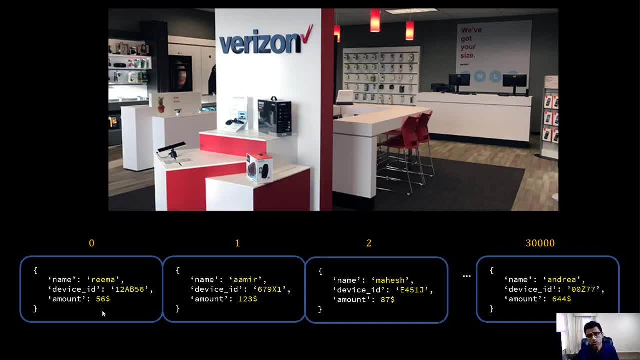 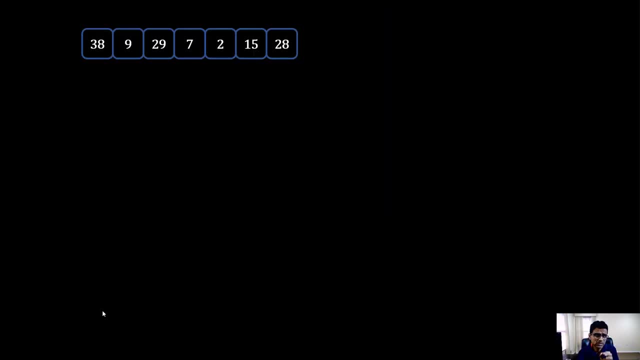 this based on a name. So sorting is a very common use case when you're doing software development and bubble sort is one of the sorting techniques. The way it works is, let's say, you have a list of numbers and you want to sort this list. 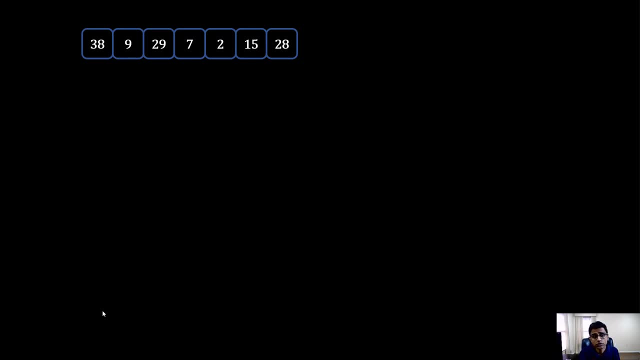 You will begin by comparing the first number with this number and the second number with this number. You will begin by comparing the first number with this number and the first number with this number. first two numbers: 38 and 9. then if 38 is greater than 9, i will swap it. so now 9 came in front of. 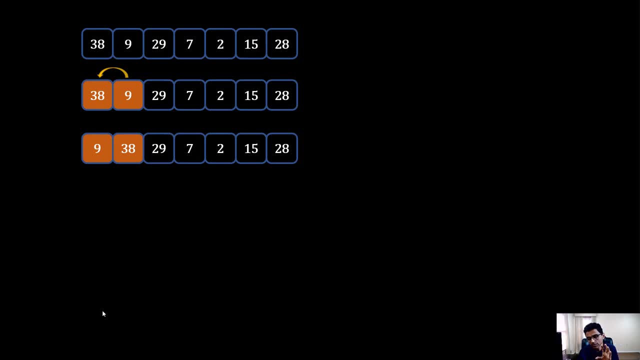 38. then i repeat this process for second and third element. so i compare 38 and 29: 29 is less than 38, so of course i will swap that, and now my list looks something like this: i again do the same process for element number three and element number four. 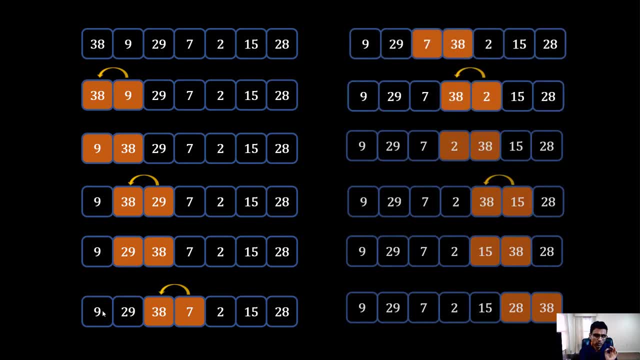 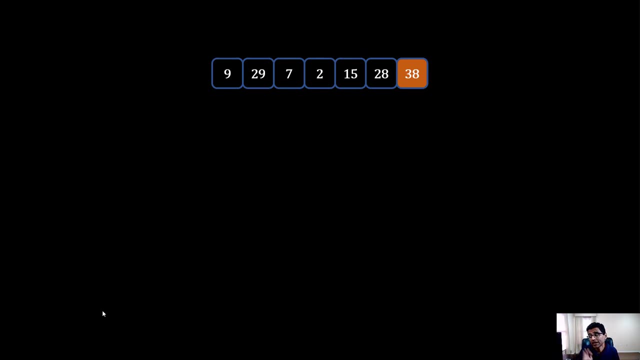 so i can keep on doing this process until the very end, and what will happen as a result of this process is 38, which was the highest number, will go towards the end. that's why this is called bubble shot, when you have a bubble in a water bubble. 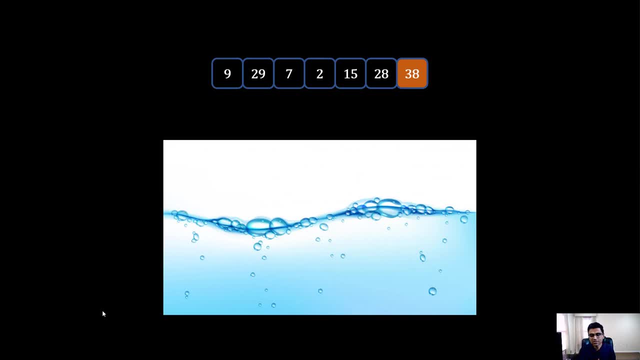 will go towards the end and that's why this is called bubble shot. when you have a bubble in a water bubble, it will pop up. it will come from the bottom to up. similarly, 38, which was the highest element, popped up from the bottom. it went all the way up to the correct position. so if you look at, 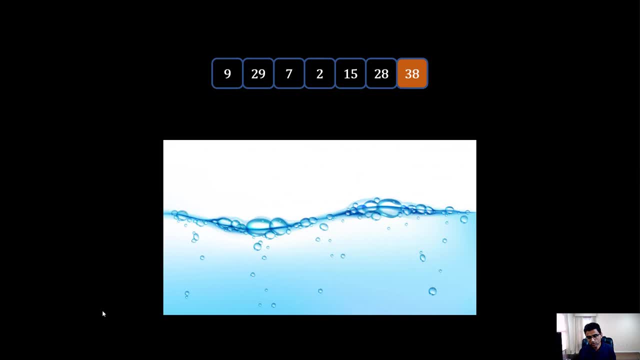 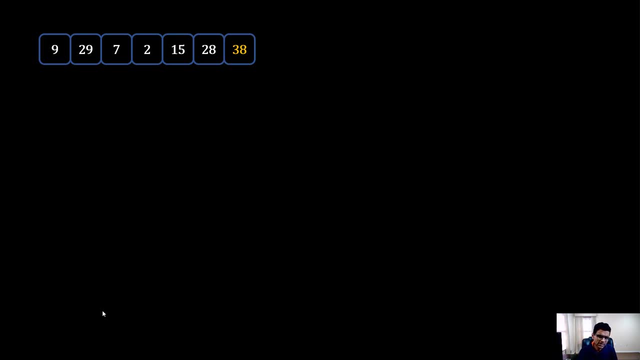 all the numbers, 38 should be in the last position because it is the highest number. now we got 38 in its right position. let's repeat the same process again. and what happens? you can literally take norton pen and you can take norton pen, and you can take norton pen and you can take norton pen. 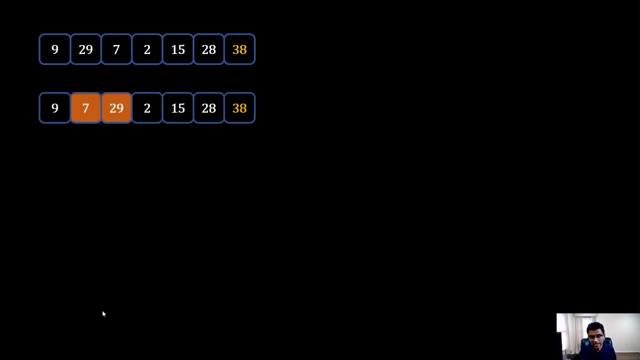 and do this process by hand. i think you should do it because that will be very helpful. so now i compare 9 and 29 and that was at the correct position, so i did not do anything. but then i compared 9, 29 and 7 and when i compare that i found 7 should be in front of 29, so i swept. 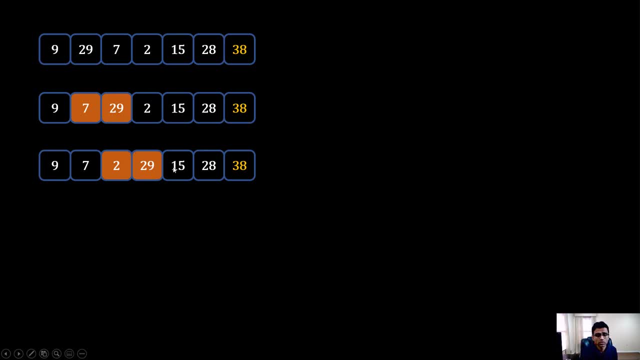 then i compare 29 and 2, then 15 and 29. so remember, what we're doing in each iteration is we come take two consecutive elements and compare, and if the first element is greater than the second, then we just change the position, we just swap them. 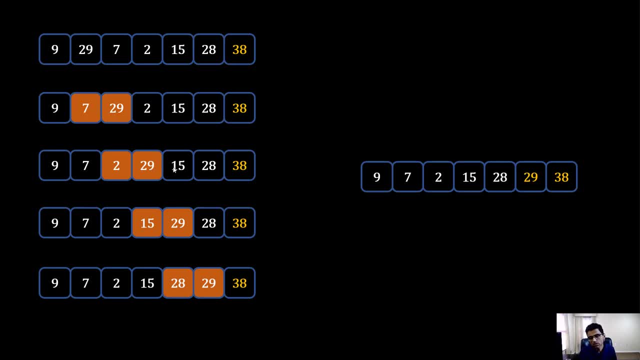 and when you do that after second iteration you got 29 in its correct position. so now, last two elements of my list are already sorted. so if i keep on doing this process for as many time as there are elements in the list, i will get my whole list sorted, if you think about. 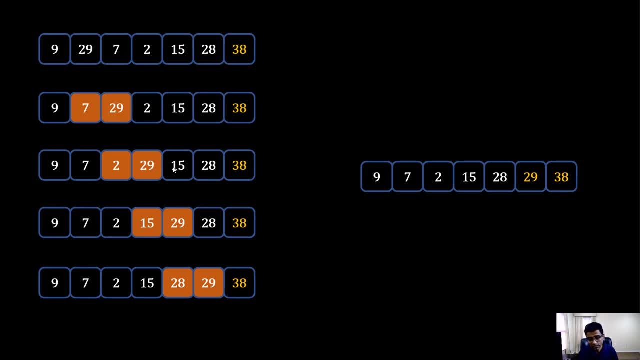 it. i don't need to do it n times. let's say n is the size of an array. i need to do it only n minus one time. i have to do this for loop for all the elements and then, within that for loop, every time. i am comparing two consecutive elements and running the second for loop. uh, throughout the list. 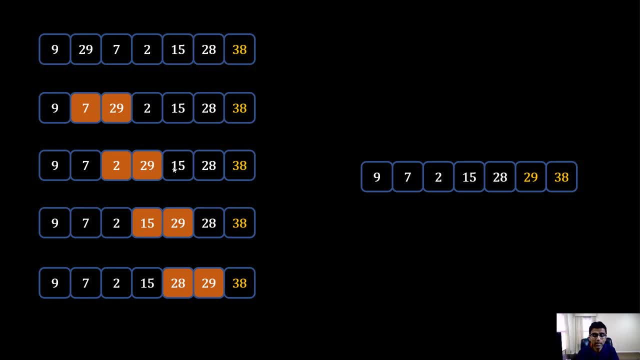 so if you have two for loops running, your bigger complexity is order of n square. if you don't know about bigger complexity, please watch my bigger notation tutorial in the same playlist. it was, i think, a second video. you'll get an idea. so time complexity here is order of n square. 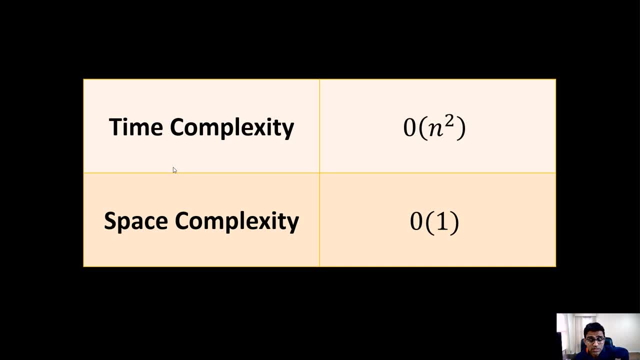 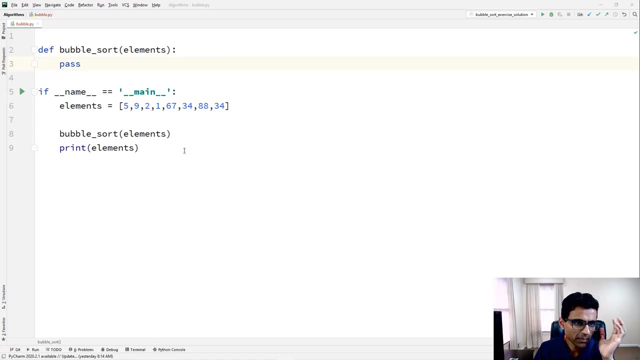 and the space complexity is order of one, because we are not using any additional space. we are just doing the same array and we are swapping the element, and for swapping the element we need some one extra variable. let's implement this in python now. in my python code i have this element: 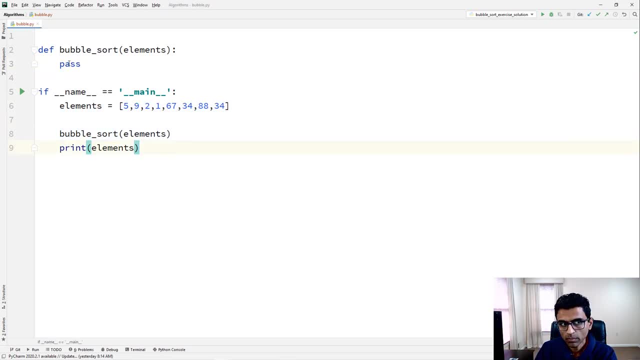 list, which i want to sort using bubble shot method. right now, method is empty and we are going to implement it as per the theory we saw in the presentation. the first thing i want to do is i want to gather the element size, because that will be very useful. 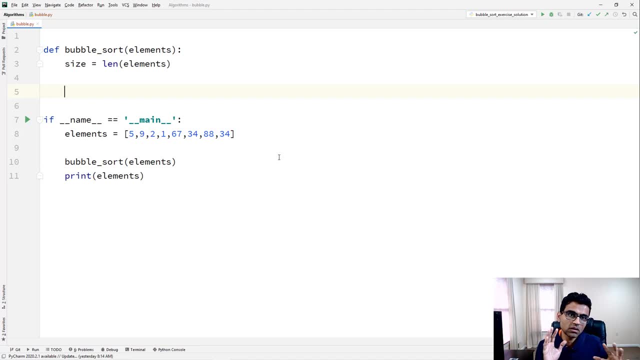 okay, and what we did- if you think about the presentation that we had- is we go through all the elements one by one and we compare consecutive elements like this two first, then this two, then this two, and so on. so how can you do that? well, you can just say, for i in range size minus one. 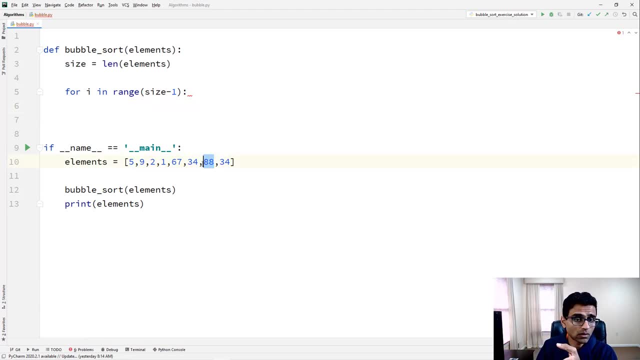 because you want to go all the way till here only because after you compare 88 and 34, there is no element after 34. hence i have minus one here. and you want to compare two consecutive elements. so let's compare them. so the first element would be what i, okay, and you want to compare that with the second element. so if i is, 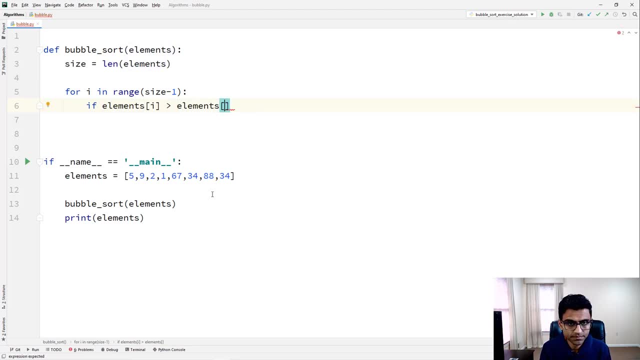 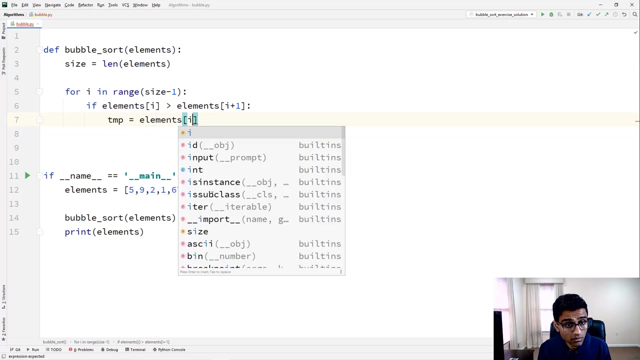 greater than i plus i plus one. okay, then you want to swap them. swat swap meaning change the position. so how do you do that? standard ways you can take a temporary variable, store elements there because i want to do this. elements i is equal to elements i plus one. 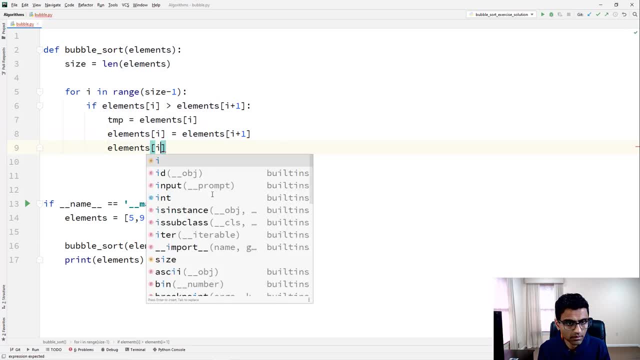 and then elements: I plus 1 is equal to. so you're doing elements this. okay, so this will be TMP and when you are done running this loop, you would have sorted the highest element. so the highest element, which is 88, will come at highest position, which is at then. so let's just run this. this code is not. 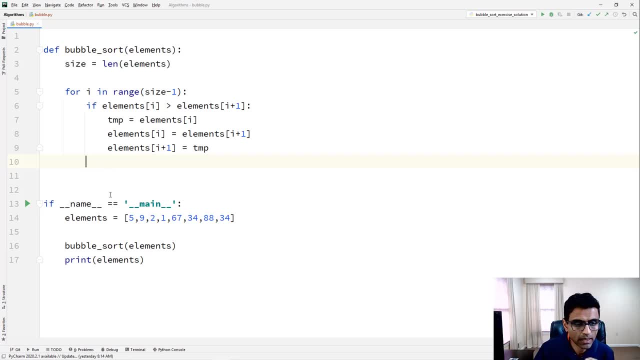 complete, I know, but I want to run it to see what happens. right click, run in pyjama and you realize that 88 came at the right position. you see, now, if I do this process two times, then the second highest element will come at the right position, which will, which is 67, let's say so. I want to keep. 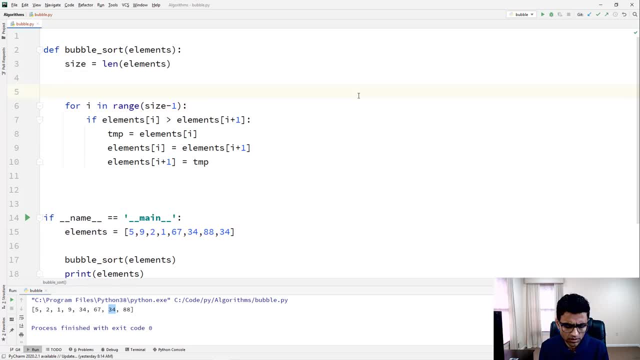 67 here. so how do I do that? well, just think about it. if you do for any loop, like for K in, let's say, range to, you're doing this two times, okay, and when you do that, you will see that 67 also came in the right position. so how many times you want to repeat this process? you want? 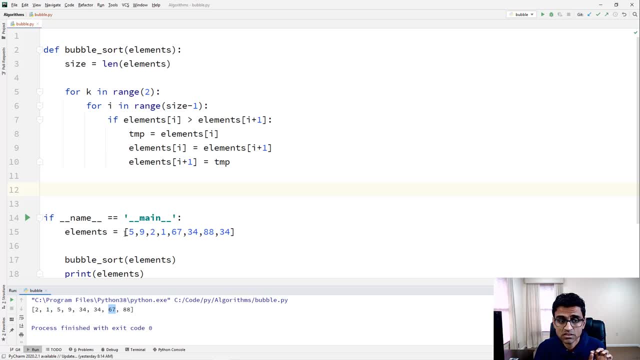 to repeat this process as many times as n minus 1. basically n is the size of the array and n minus 1, because when you repeat process two times, you get two maximum numbers in the right position. similarly, I want to get all this number in the right position and the first number will. 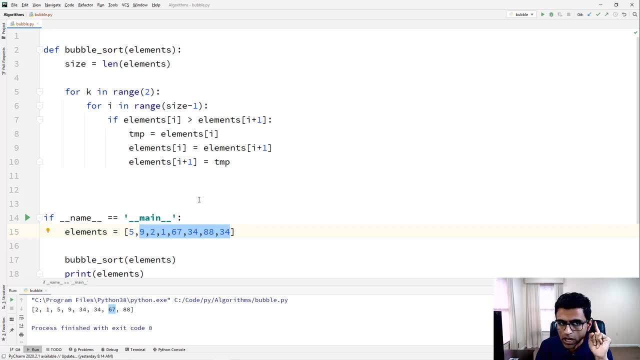 automatically come into the right position. okay, so the outer loop. so also, let me just change this inner loop to call it J. okay, I'm just changing the loop variable and nothing else, because this is a standard convention we have. so I'm just calling it J. out outside loop. I am calling. 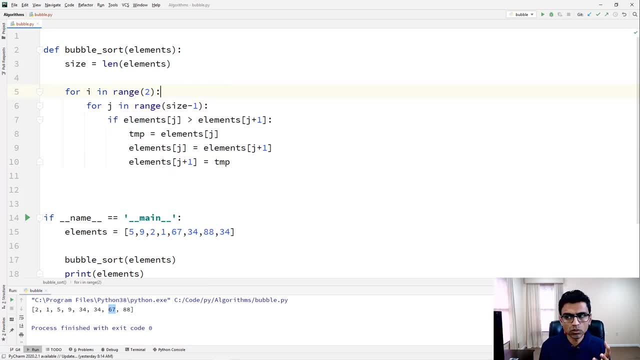 it I and I want to run this loop for size minus 1. I hope it makes sense. it's pretty simple actually. when you run this code, you will notice the whole list is sorted now. this process is probably not the most efficient, because this see, we are, we are. 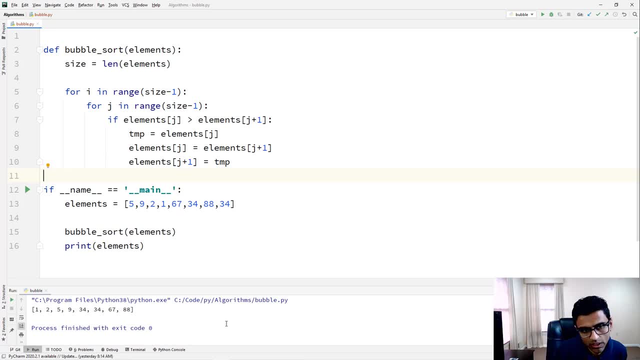 having couple of inefficiencies. okay, so what is that? when you ran this loop for two times and, let's say, last two elements were in the right position, third time, when you run the loop, you need to run it only till this point. you can ignore the last two elements because they are already sorted. and the way to ignore that would: 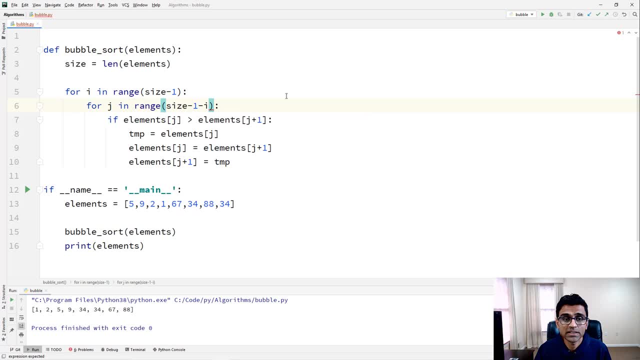 be here. you can do minus i, so minus i will be when you are in second iteration. you don't go all the way to land, you go all the way till n minus two elements. okay, that way you save some time. basically, on iteration, right now code is running very fast, but when you have bigger, less, 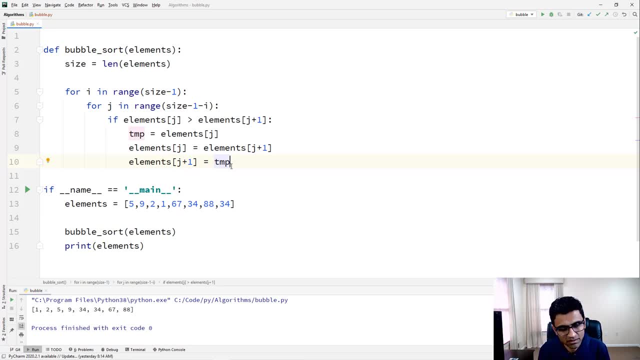 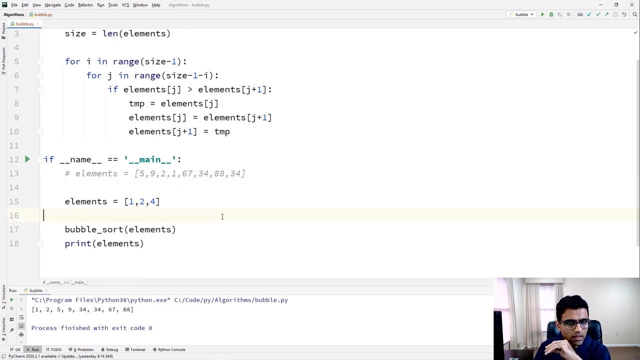 a million elements. save some time, some millisecond also, let's, let's do this. okay, let me run this for already a sorted array. so let's say, this array is already sorted and when I run it, of course it's gonna remain sorted, but what will happen is I set a 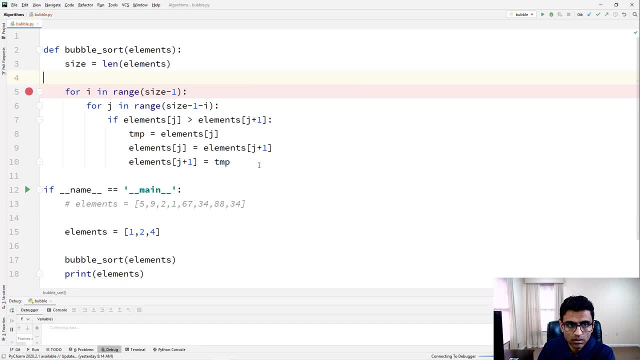 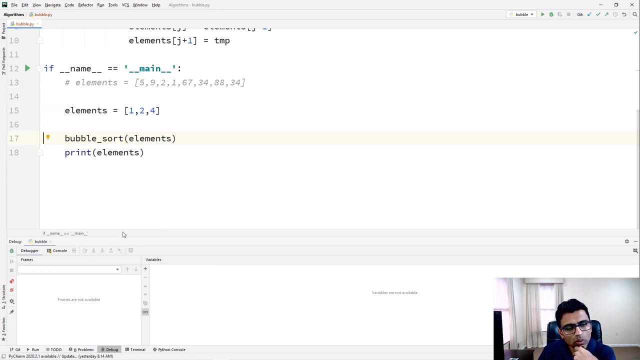 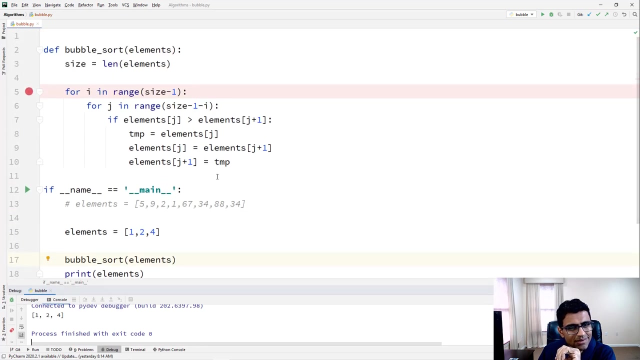 brick breakpoint here, or right click debug- okay. and when I go to next point, see it keeps on repeating this loop, although the array is sorted. is there a way to detect that array sorted? yes, there is a way. think about it in your inner loop. let's say, if you go through, 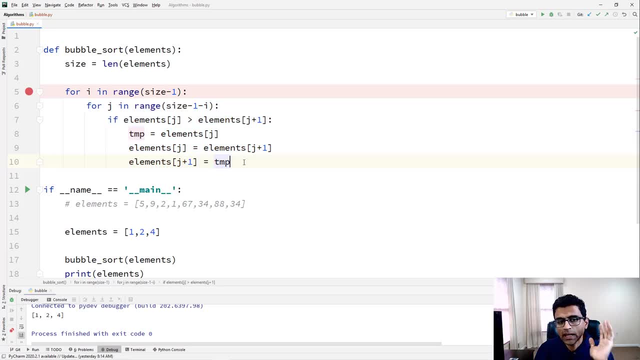 the inner loop. let's say, if you go through the entire list and if you don't end up swapping any element, it means your array sorted. so here we can create a variable called swap which is false, and whenever you are swapping you just say swap is equal to true and what we'll do it you. 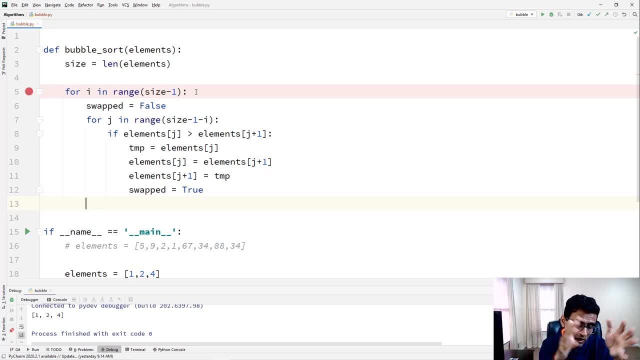 will do is your inner loop after completion completing, if it has not swept an element, the swap flag will be false. okay, so you can say: if not swept, break now you can break the outer loop. okay, and this will make your algorithm more efficient. we can verify it. so, if I debug, 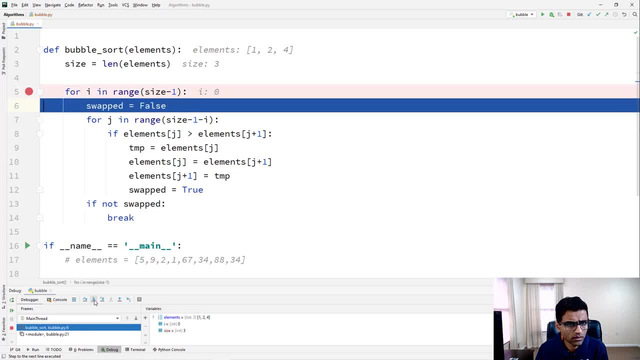 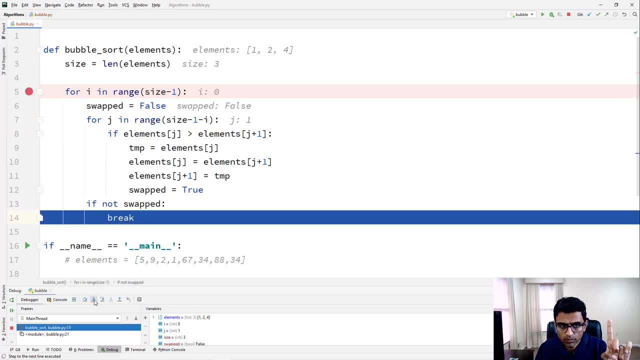 here and if I go here, see outer loop, I am, you know, my first iteration. okay, inner loop, see in my outer loop. I just did one iteration and I'm I'm done now. so the complexity of this will be: order of n. it is not order of n square, because you. 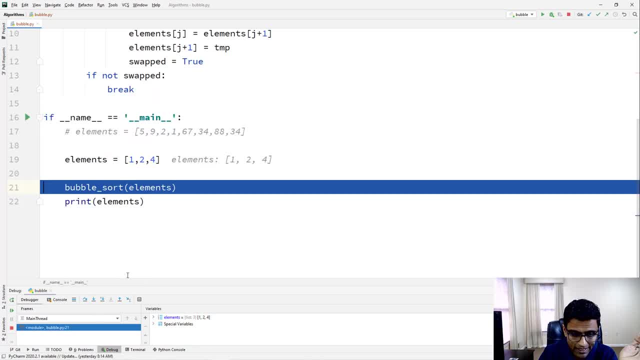 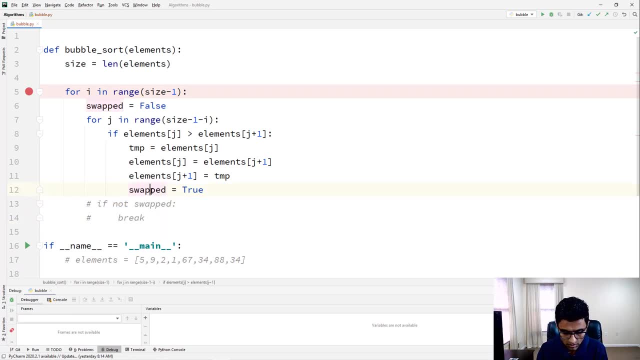 went through the list only one time. if you don't have this code, let's say I don't have this code here, okay, without this code, what? what was happening? you might have realized it. you start with the outer loop, the first iteration, then you go through all the 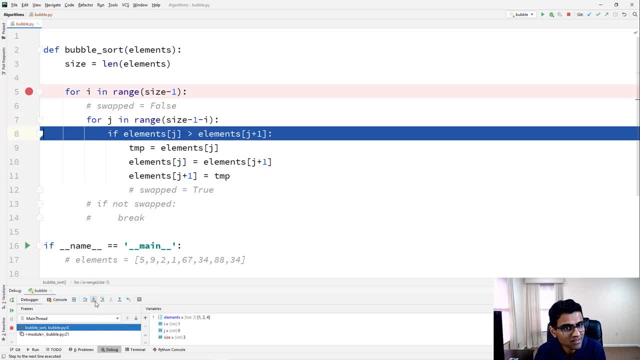 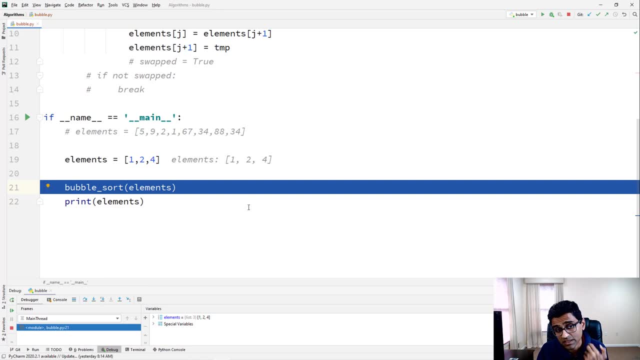 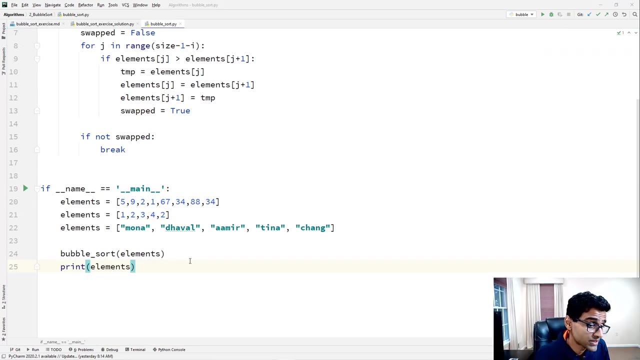 elements. now see, you are in a second iteration. this is not needed. then you go through all the element, you go to third iteration. so all of that was not needed, and this can be made efficient by using this swap flag. by the way, you can use this sorting algorithm to sort the strings too. for example, I have this list: 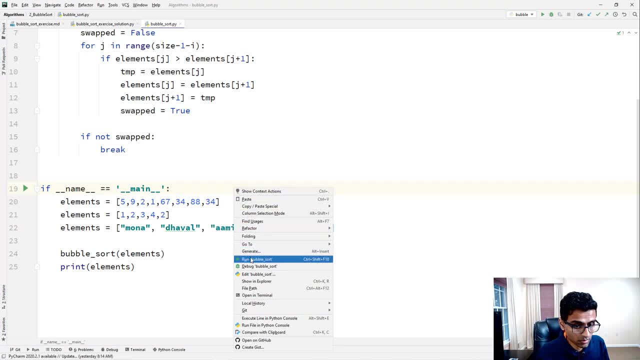 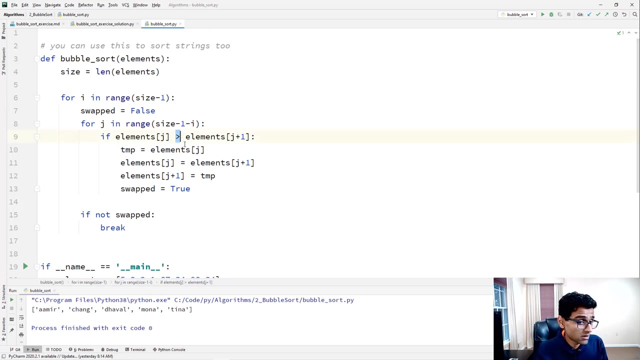 of string and when I call bubble short on top of it when I run it you see these are alphabetically sorted. now a comes first, then C, then D and so on. this is because in Python you can use this greater than operator on strings. you can quickly verify it if you say a is greater than. 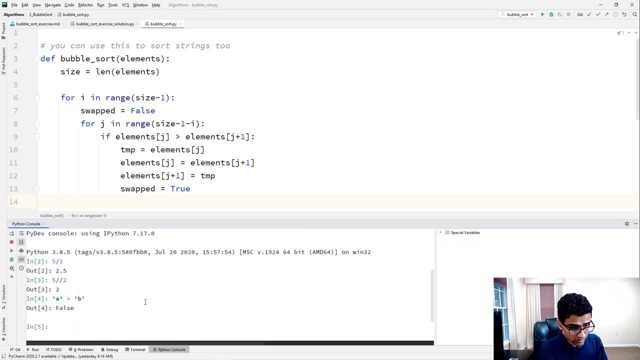 B, It returns false. But if you say a is less than B, It returns true. Similarly, it does the comparison for the whole string as well. For example, you have ABC and you have ADX, It will return true. Alright, so that's all I had for. 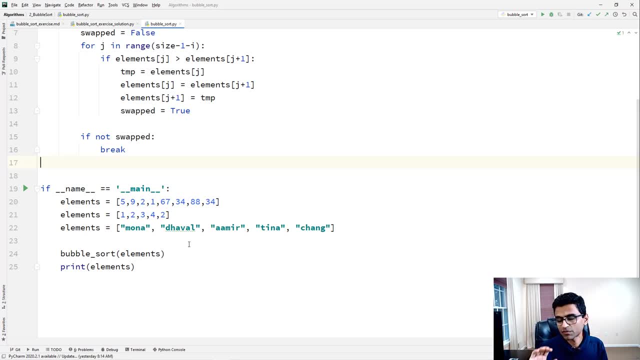 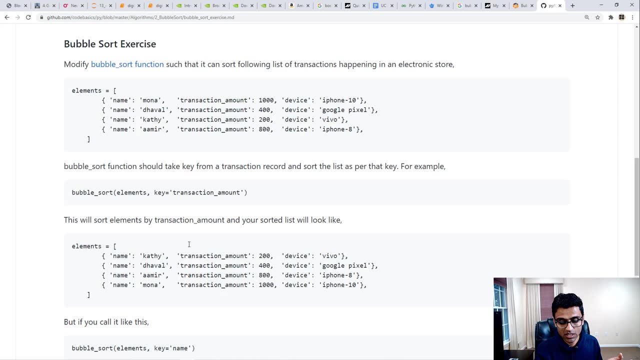 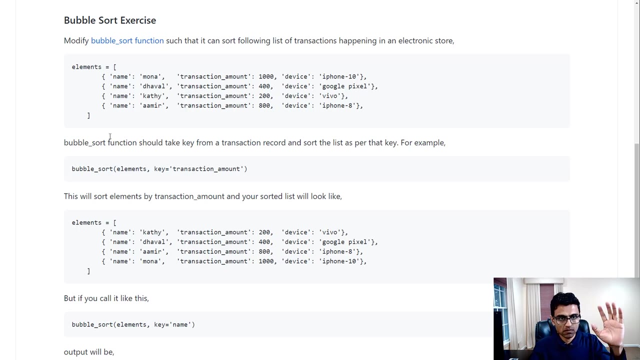 Bubble short and now comes the most interesting part of this tutorial, which is an exercise. you cannot learn things unless you practice on your own and you Do this exercise. so I have this interesting exercise for you, where I have the transaction records of electronic store and I want you to modify my bubble sort function to take a key argument. 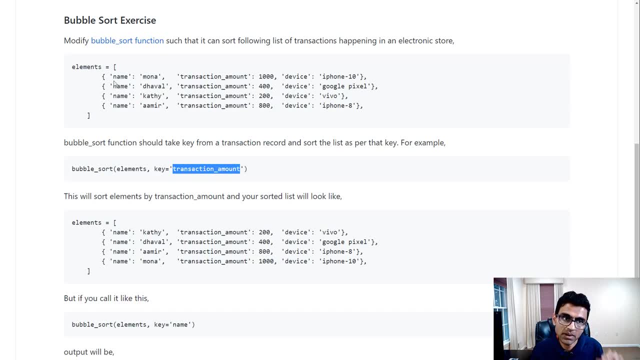 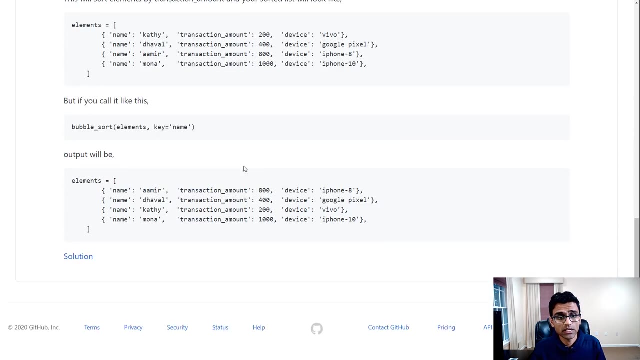 where I can specify a key inside my dictionary and Using that key, It should do shorting. For example, if I say My key is transaction amount, then it has sorted all these records by transaction amount. You can see two hundred four hundred eight hundred thousand. if I say key is equal to name, it will sort them using the names. 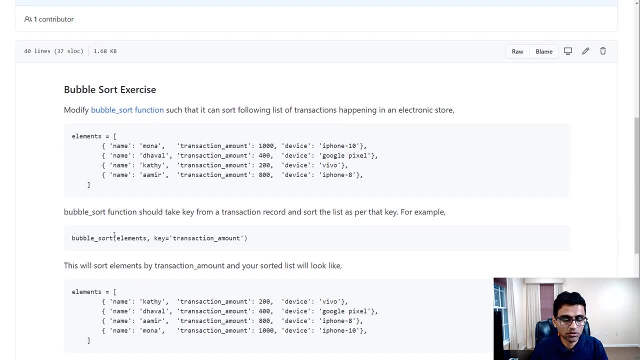 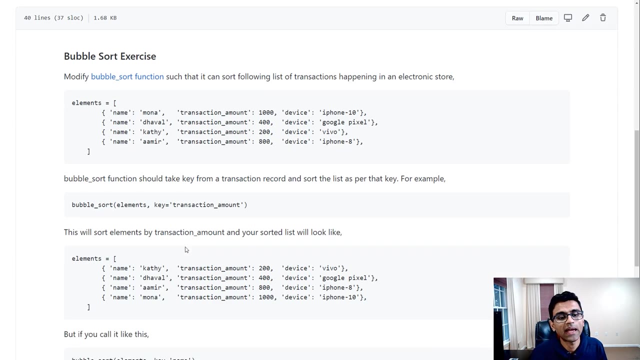 the solution is actually simple. you have to just Take my function- by the way, I'm gonna provide my Jupyter notebook in the video description below, So make sure you check the video description. It has a link of this exercise as well- and and you take my function, add this key element and then, when you are doing that comparison, you know.